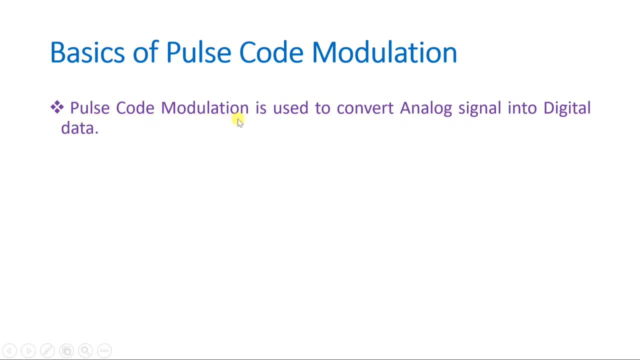 And for that this is very popular method, which is what we are using: it to convert voice signal into digital data And in that first we will be doing sampling to convert that given analog data into discrete analog signal. Like see, if you have one signal which is continuous analog signal, then by having the sampling 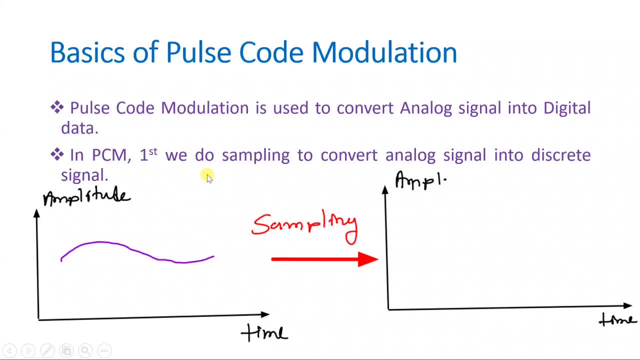 we can convert that into discrete signal and even I have made all the sessions regarding sampling in this playlist of digital communication. you can go through it. After sampling, we do quantization and this quantization is being done to convert given discrete signal into digital signal where you will be finding there are predefined quantized 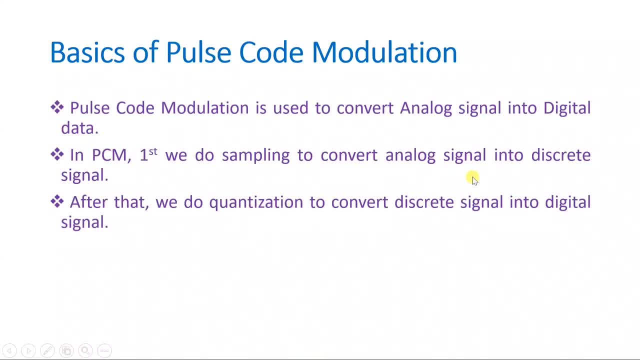 level will be there And we will be translating that discrete sample, Quantized samples, into predefined digital samples and after that we do encoding so that encoding will translate quantized samples into digital data. So this is the basic thing which we do it in Pulse Code Modulation. 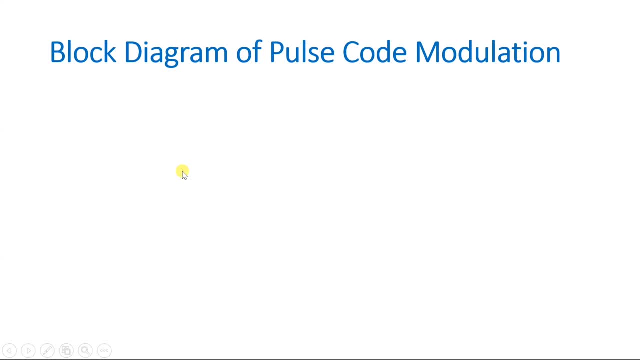 Now let us try to understand all those things by block diagram and by waveforms. So see, we have analog input over here, So you can see here continuous time analog input that we have Now, this input that will be given to sampling, So we will be having sampled output. 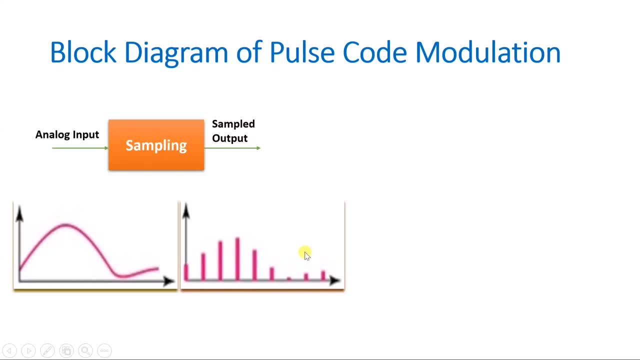 In my previous sessions you can see I have explained sampling as well, as there are different types of methods of sampling where we can have ideal sampling, natural sampling and flat top sampling. So out of those we can use any method, Any method to convert given analog signal into discrete sampled output. 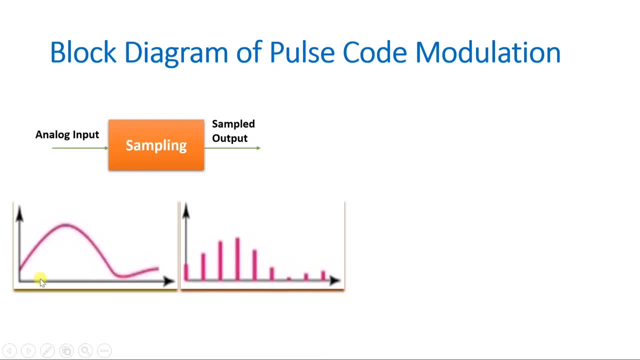 So here in sampling we choose sampling frequency, So at fixed time interval we will be having a samples. you can see Now this sampled output that will be given to quantizer. So quantizer will quantized this sampled data And it will be. 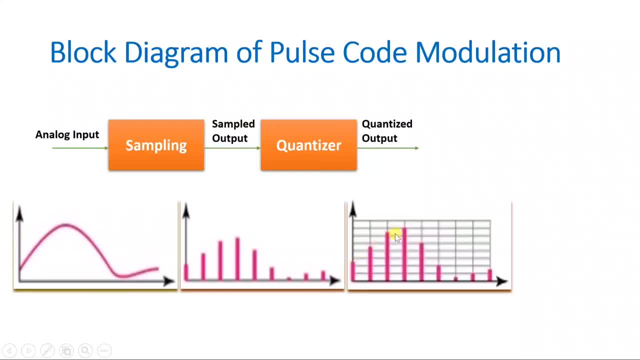 Converting this data into predefined sets of values. So what? based on approximation and few sets of rules, we convert this sampled output into quantized output. So in quantized output there will be fixed levels. you can see. See, in sampled output, amplitude will be continuous. there will be no fixed data, which is there. 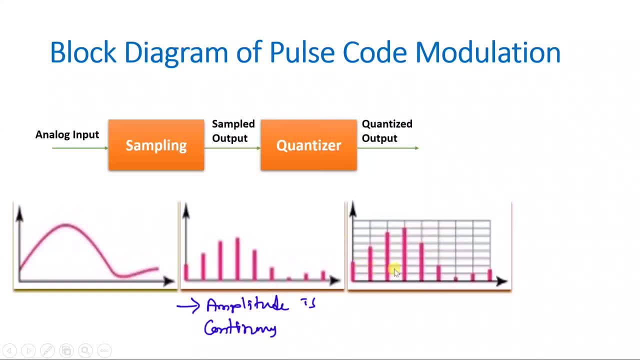 with samples. But once you do quantization there will be fixed intervals and those fixed interval that will be assigned to particular value, which is there with sampled output. So for example, you can see this sample that is assigned with this amount of amplitude in quantizer. second is given with this amplitude. so likewise we give sampled output to quantizer. 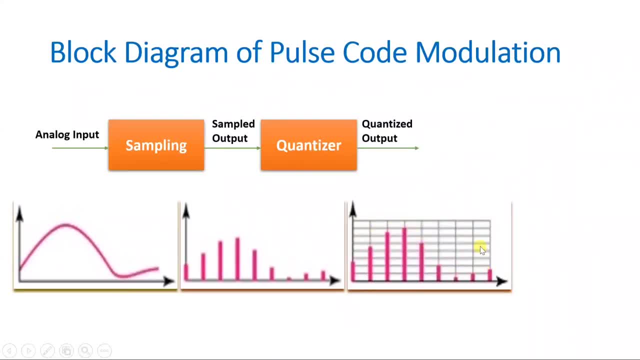 and it will be converting into fixed values. So here, for example, if I say I have three bits to represent given data, So three bits can have total number of samples that is equals to two to the power three, So total eight number of samples are there which can be used to convert this sampled. 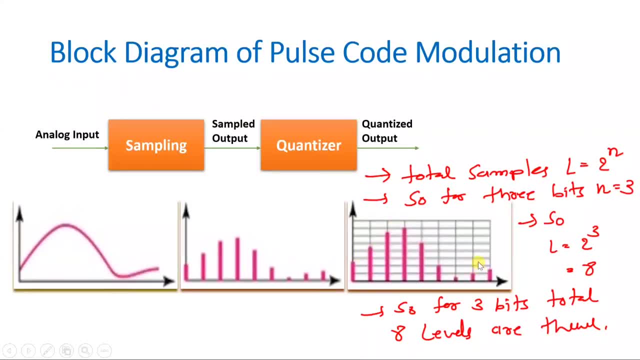 signal into quantized signal. So here you can see There are total eight levels. So here there are only eight possible amplitudes to which we will be giving amplitude right Now. once we have this quantized data, then by having encoding we can convert that into. 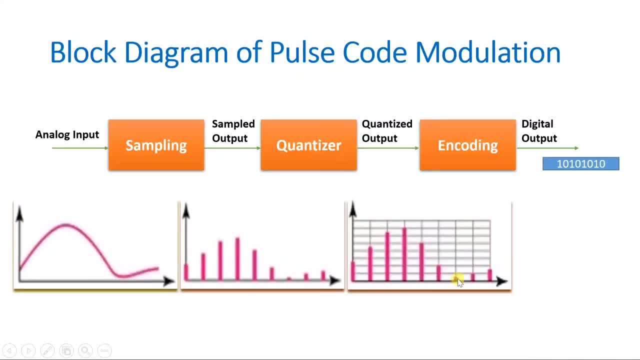 digital. like: see, if I say this first level, that is, having zero, zero, zero data, then second level is having zero, zero, one third is having zero, one zero. We can assign direct digital data to quantized signal and this digital data that is what we can carry for further communication. 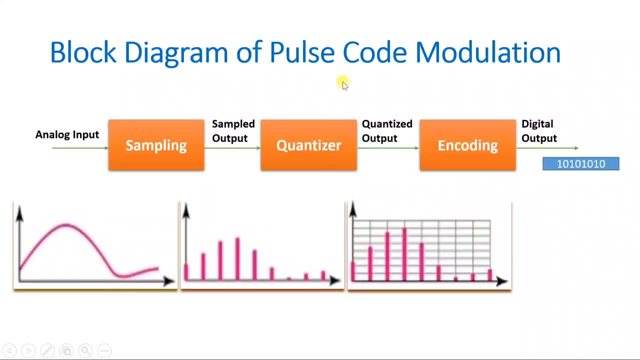 So, ultimately, this is what complete process, which we do it in pulse code modulation, to translate analog input into digital output. Now here are a few more things that we need to take care of. One is If, At input side, frequent high frequency components are there. in that case, 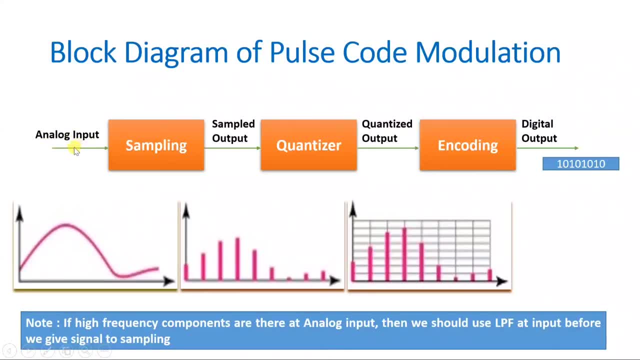 We need to place low pass filter over here before we give it to sampling. So if you provide low pass filter over here, then that will eliminate high frequency components, which is there in analog input, And in that case we will not be having any sampling error as we have removed high frequency. 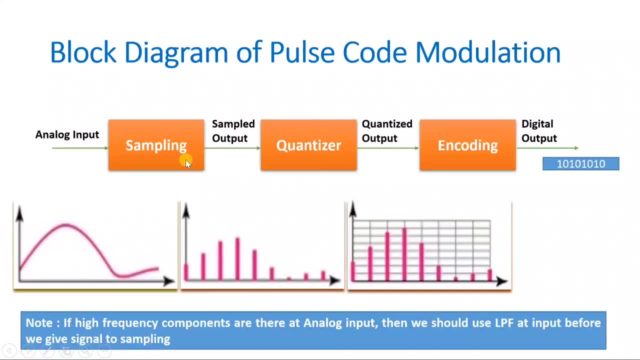 components And even sampling is being done based on what is maximum frequency, which is there at input side, So it should not have very high frequency to avoid sampling noise. So there is a possibility of analyzing as if we don't provide sufficient sampling frequency. 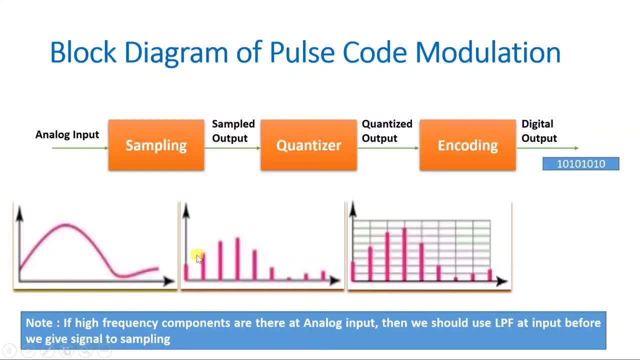 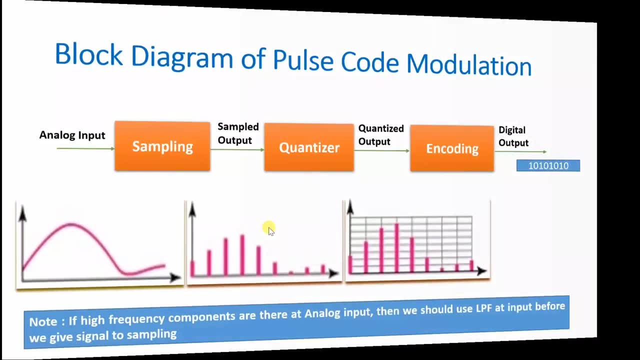 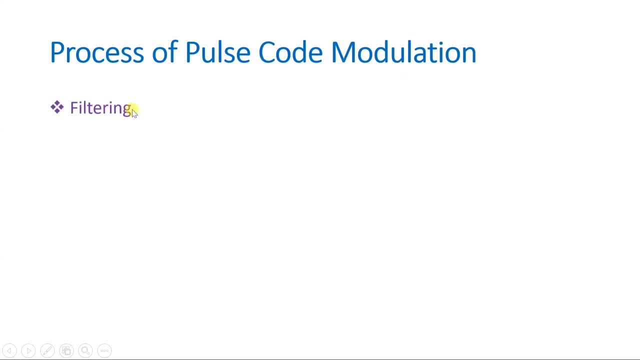 And as if you increase sampling frequency, in that case there will be issue regarding bandwidth, So That we will see step by step. So now see process of pulse code modulation. So where first we do filtering operation and that is what we do it at input side, where 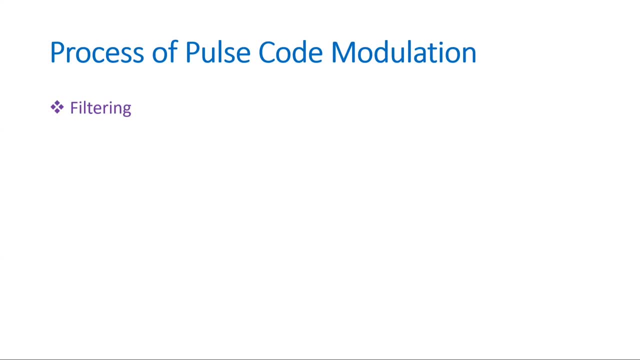 if we have some high frequency components in input signal. in that case, by using low pass filter we can eliminate high frequency components and after that we give it to sampling where. So that sampling frequency is so essential in sampling, that justifies bandwidth of pulse code modulation. 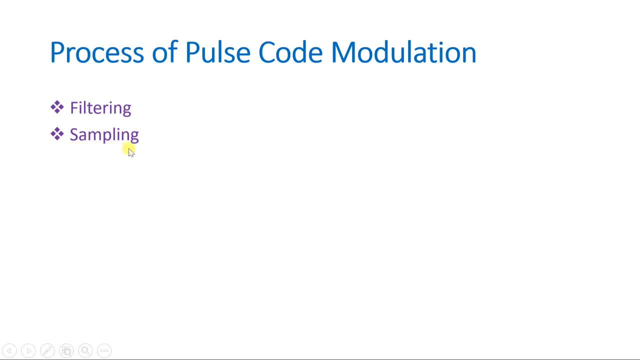 So even how to calculate bandwidth and how to calculate data rate that even we have delivered to see later, Then, after we do quantization, where discrete signal will be converted into quantized signal and that quantized data is now ready to encode. So after encoding we will be having digital. 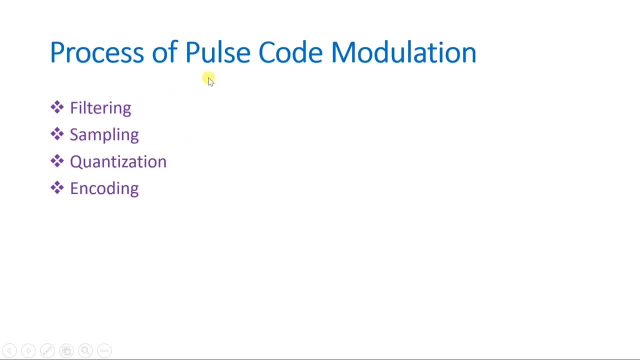 So this is the basic process which we do it in pulse code modulation. Now let us see all those things step by step. So see, we will see first sampling in pulse code modulation and this is what we are doing: it to convert continuous analog signal into discrete signal. 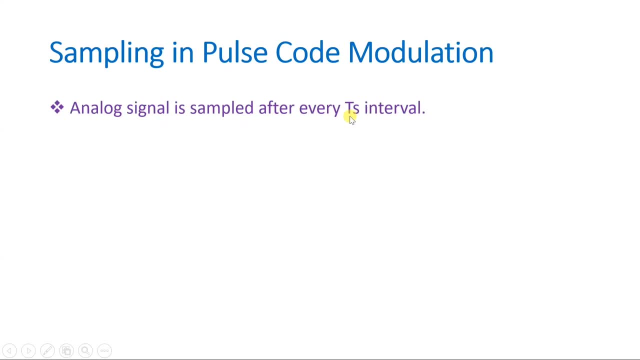 And discretization has been done with respect to time interval TS. that is even referred as In this section. this can be modified later. skip to 7 for sampling time interval. So now let us take our sample in pulse code modulation, which we just did in phase C 2. 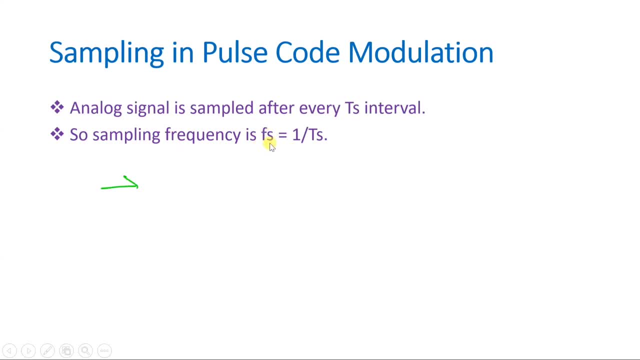 basel, shear mapping, essentially. So we have one noise DILED, surprised, bring energy to output, and one noise B hdd is tensed, as we did now with every field, F, g, r device radically modified and its nevertheless amazing length as well. We also lines tonez ass in dz. p less should be equal to the value of zero times to n. 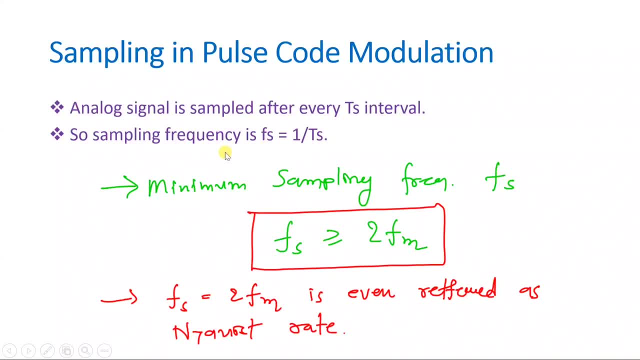 which we did already during the example that we were creating요. So after changelética, an example: another matrix for sampling time range can be created where fm is maximum frequency present in analog input. and if you don't do this, in that case there will be no reconstruction of analog data, which is 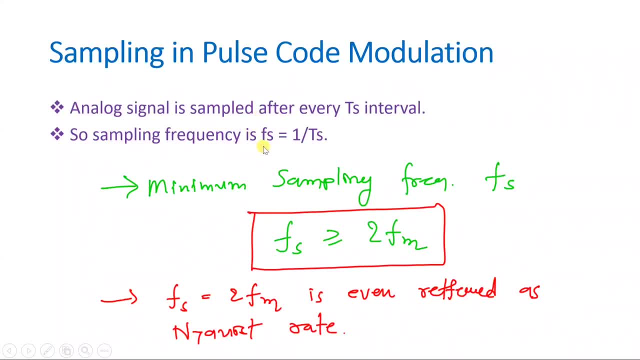 there at input side. so to reconstruct signal after having a sampling fs should be greater than or equal to 2fm. there are three basic sampling methods and I already have made separate session for all three methods. first is ideal sampling and in ideal sampling you will be finding impulses are there at each. 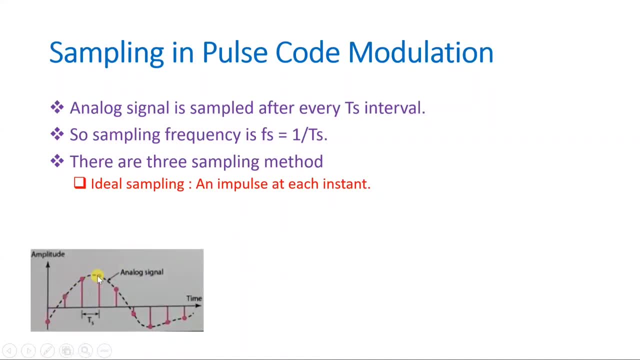 instant so you can see. if my analog signal is this, you can observe then if I provide sampling over here at instant sampling, in that case you will be finding: see at particular instant only there will be samples right and time period in between. two sample is sampling time period ts and 1 by ts, that is sampling frequency. 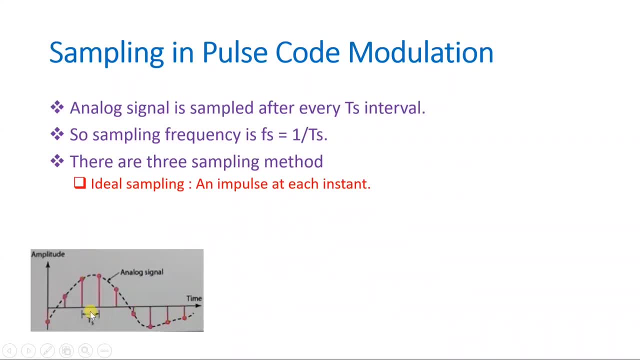 and this sampling frequency should be greater than or equal to 2 fm. now if we see second method, so that is natural sampling method, where in natural sampling method pulse of short width with varying amplitude will be there. so if you see that by this diagram, this is what my analog signal. 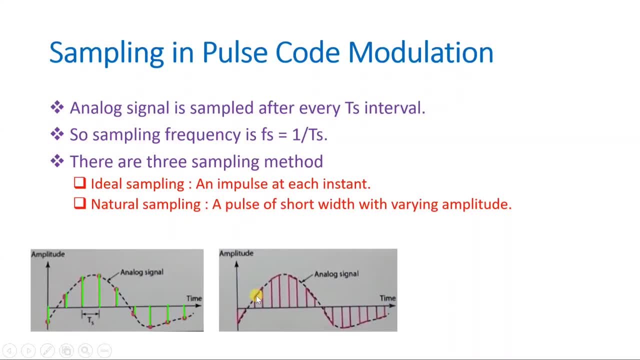 and this is my pulse. but if you observe pulse width, amplitude is varying. you can see, with this pulse even, you can see amplitude is varying, right? so in natural sampling pulse width will be fixed but its amplitude will vary, as you can see it in this waveform. now, third sampling method, that is, flat top sampling method, where 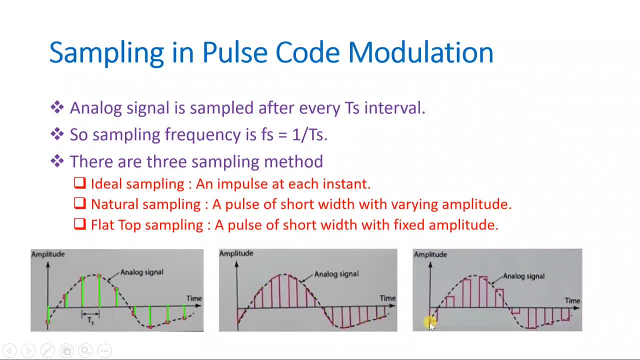 pulse of short width will be there, but its amplitude will be fixed, and this is what flat top sampling and this is what happening based on sample and hold output. and to understand all these three methods, I have made separate session for it. you can go through my playlist where, in sampling, I have explained all three. 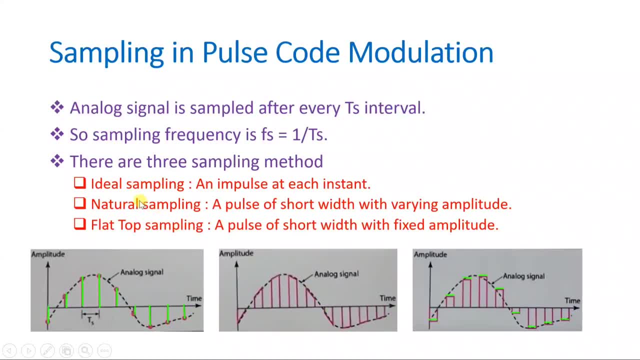 methods in detail and this is how waveforms are appearing in different sampling methods. now, once you do sampling at output side, there will be sampled output where you will be finding there will be pulses with deep finite output and there will be pulses with finite output and there will be pulses. 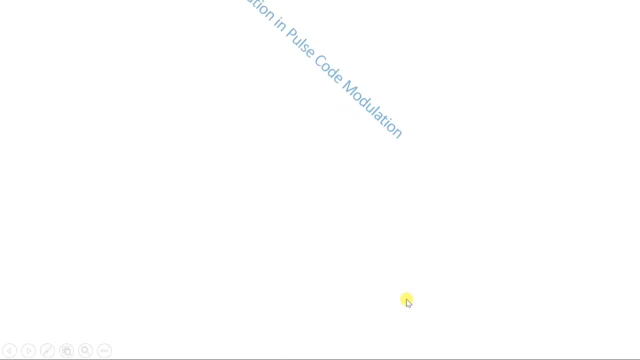 amount of amplitude and those pulses with finite amount of amplitude will be given to quantization. Now see in quantization we are dealing with to approximate values, which is predefined. So see the process of measuring numerical values of samples and giving them a table value in 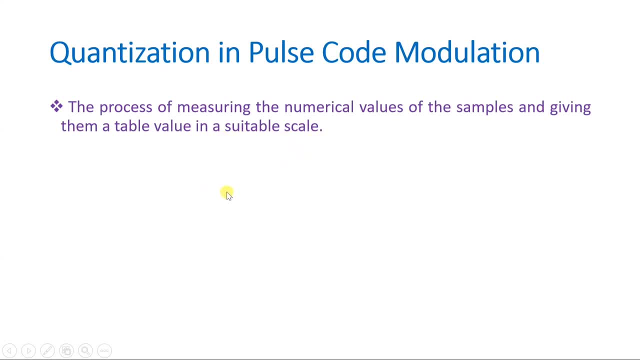 suitable scale. So, for example, if I say my amplitude is varying from 0 to 1 voltage and if I represent that by 3 bits, then total number of levels to assign given sampled output to quantized output will be 2 to the power 3, so that will be 8.. 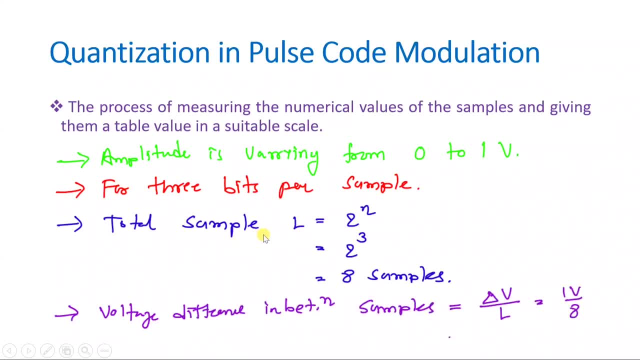 So with 0 voltage, I'll assign 0 0, 0 digital data. with 0 voltage, I'll assign 0 0, 0 digital data. So with 0 voltage, I'll assign 0 0, 0 digital data, With voltage 0. and as 1 voltage is divided into 8 different levels, second level will appear. 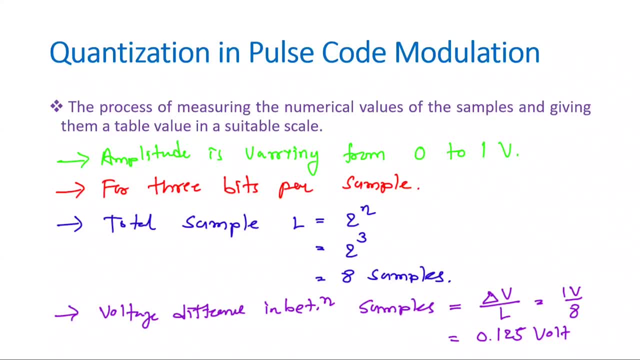 at 0.125 voltage and with the gap of 0.125 voltage, next level will appear. So likewise, we'll be finding there are total 8 levels which will be defining values of voltage varying from 0 to 1 voltage, So the finite number of amplitude of interval. 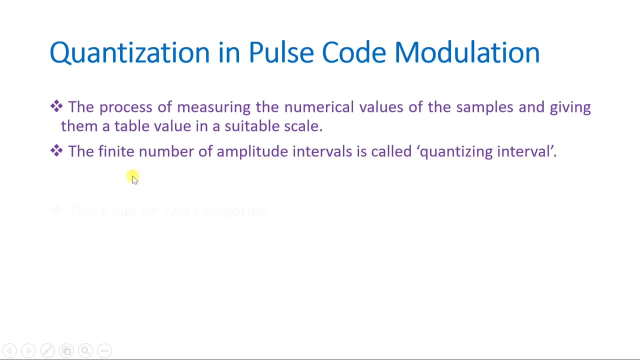 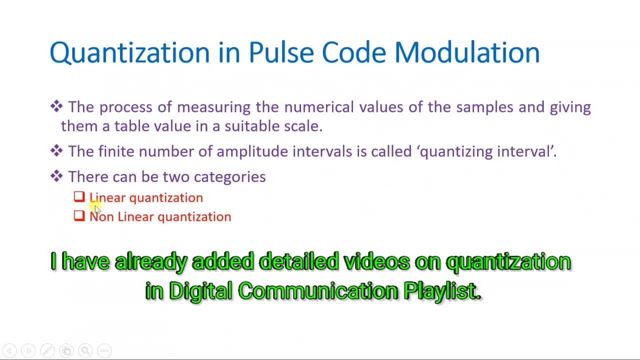 is referred as quantizing interval. There can be two categories: linear quantization and nonlinear quantization, And even in my future videos you can study both in detail Here. I'll just give you basic idea. like see in linear quantization, level interval will be at: 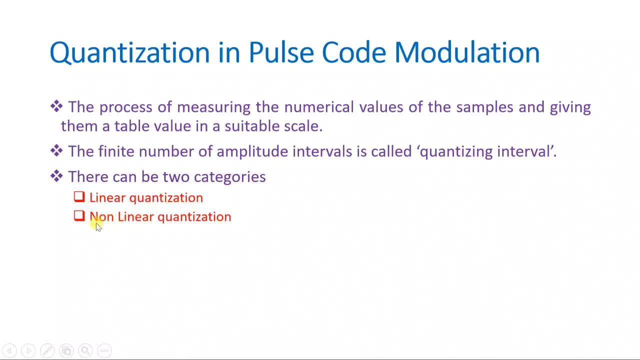 finite and fixed value. while in nonlinear quantization level of interval will be at finite and fixed value. while in nonlinear quantization level of interval will be at with respect to variation, so it is not constant. So in linear quantization we can say: see if voltage is varying from 0 to. 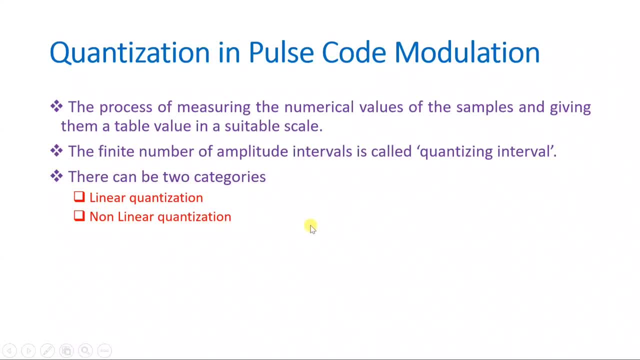 1 with 3 bit resultant, and in that case total numbers of levels will be: l equals to 2. to the power, 3 means 8 levels are there, while in nonlinear quantization levels will not appear at finite intervals. but we'reИi gonna also refer to all levels with nonlinear quantization wird. 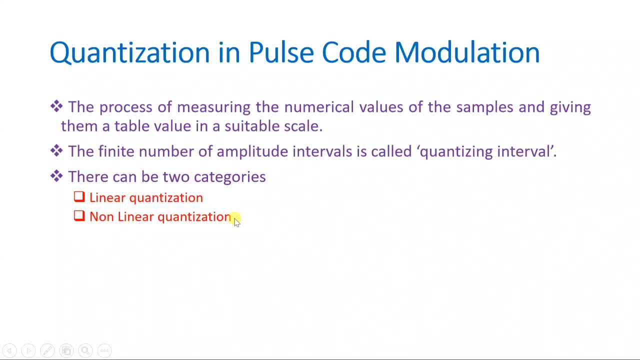 W, whether, but in any case you follow what or what kind of increases that will give in Dollars, mark and status behaviors. finite interval: it may have different values of amplitude with different intervals. so difference in between sampled output and quantized output is quantization distortion, like see for example. 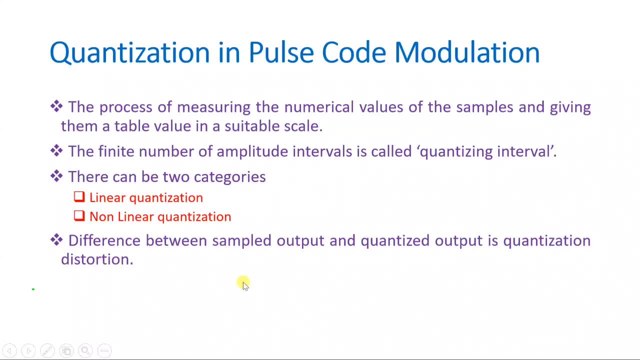 if my sampled output is 0.129 voltage but after approximation my quantized output is 0.125 voltage, which is predefined, then the difference in between these two, that is quantization distortion. so you will be finding, in this particular case it will be 0.129 minus 0.125, that is equals to 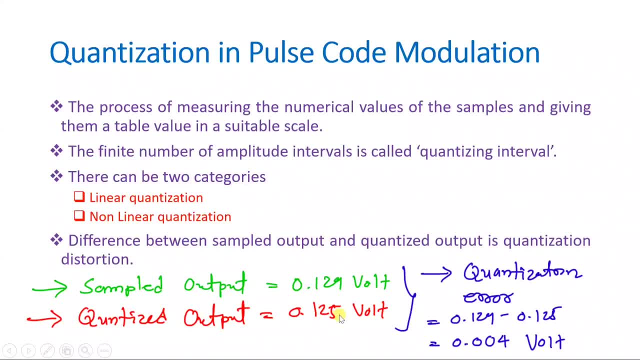 0.004 voltage. so that is how quantization distortion is appearing. if you want to reduce quantization distortion, then you will have to increase number of levels. and if you increase number of levels, then to represent given sample we need more number of bits. and if you increase 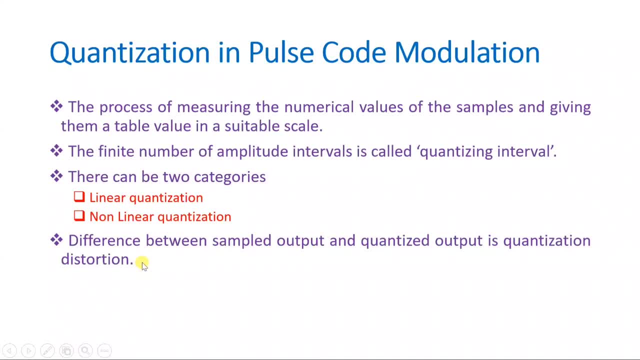 more number of bits then you will have to need, then you will have to have more bandwidth to transmit data. so to decrease this distortion we can increase number of levels by increasing number of bits. so this is what the basics, which is there with quantization. now let us see the standards, which is there with pulse. 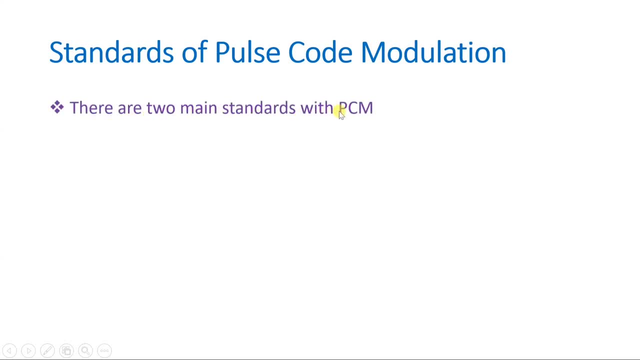 code modulation. see, there are main two standards: which is there with PCM and this is what we are using it in digital audio data, and those two standards are there with European standards and with American standards. so these are the two major standards which is there with pulse code modulation to digitize audio. 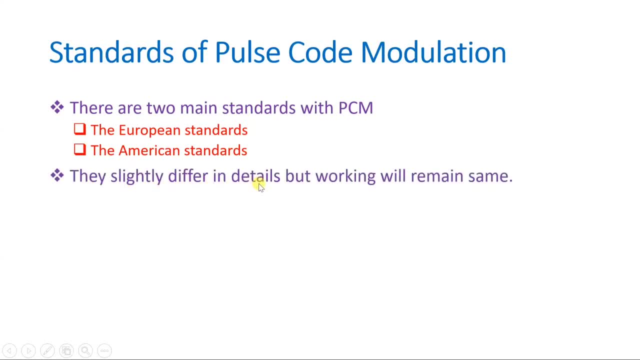 signal their site slightly differ in details, but working will remain same. so working is same and that is what we have already seen. in terms of details, it will be bit different. European PCM is having 30 channels and North American PCM is having 24 channels. Japanese PCM is having 24 channels and in India, 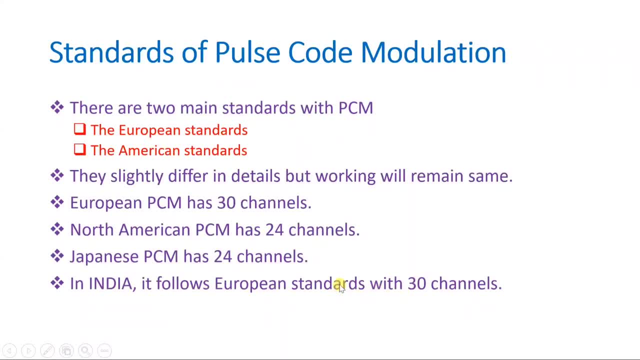 we follows European standards with 30 channel. so there are major two standards: European standards and standards, and in India we follow European standards with 30 channel. here I am not going to show you all the details regarding all those PCM standards for that. in future I'll make separate session for that. now, how to calculate. 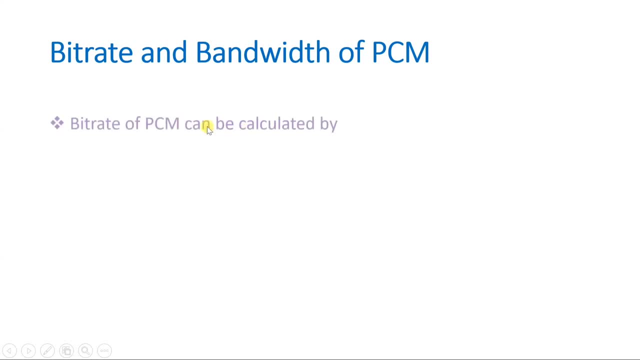 bitrate and bandwidth of PCM. when we talk about PCM with voice of the subject, now we have to calculate bitrate and bandwidth of PCM. when we talk about PCM, now we have to calculate bitrate and bandwidth of PCM. when we talk about PCM- bandwidth and bitrate- then bitrate will be based on sampling frequency and number of bits required. 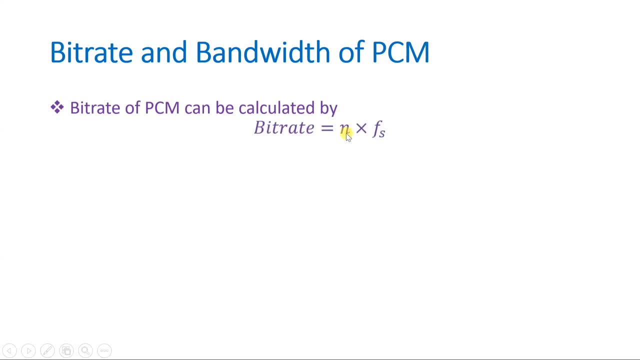 to represent sample. so bitrate will be n into fs, where n is number of bits required to represent one sample and fs is sampling frequency, now bandwidth of pcm. that depends on which type of encoding is being done. so once you identify bitrate, then that data rate will be encoded. 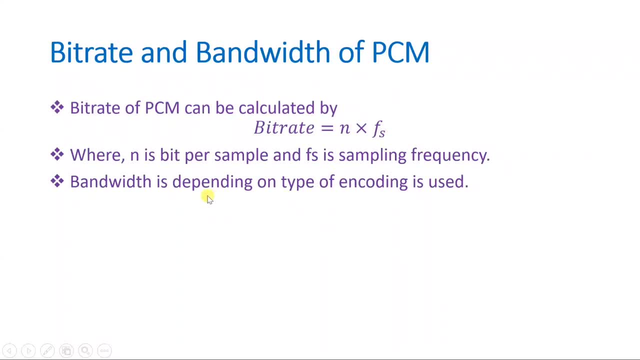 in particular scheme so that scheme might be having some finite bandwidth and as per that we'll be having resultant bandwidth of pcm. so bandwidth is depending on type of encoding that has been used and from bandwidth will even come from bitrate- only right, so bitrate can be calculated directly like an integer. 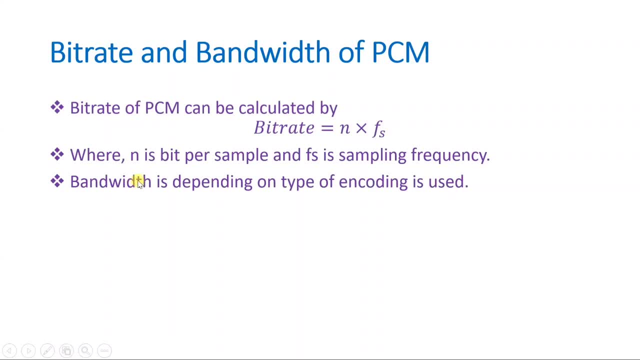 to fs, but bandwidth that is also depending on encoding scheme. so digital signal requires more bandwidth. but we pay price for robustness and digital communication. there are many advantages, which is there with digital communication, so we convert analog signal into digital and then we do digital communication because of so many advantages, and already i have explained many advantages. 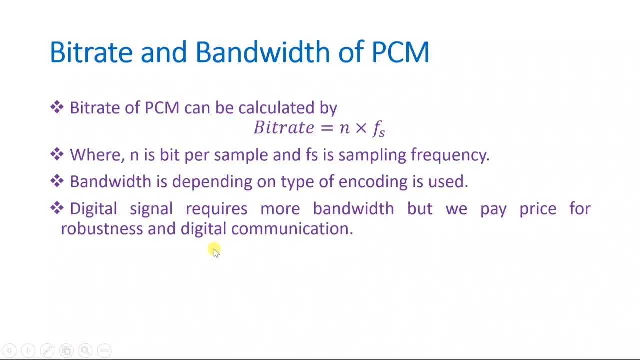 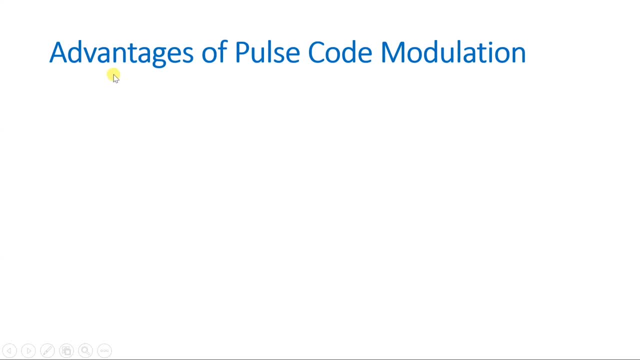 of digital communication in initial videos of this playlist. now let us see the advantages which is there with pulse code modulation. uniform transmission quality can be maintained by having a pulse code modulation and compatibility of different class of traffic in network can be assigned. like see, if you use text data, that will 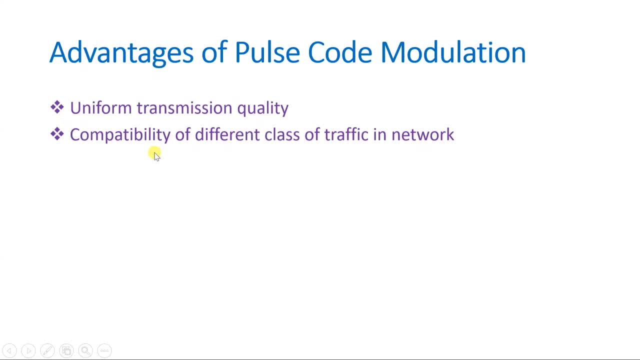 be digital. if you use video data, that will be digital and in parallel with that, by converting audio signal into digital, we can have compatibility of different class of traffic in a same network. so this is what possible due to pcm. integrated digital network is utilizing that facility of voice translation into digital.